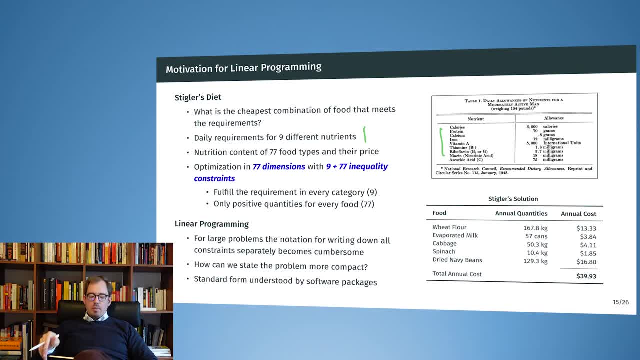 For the 77 food types, we can add the constraint that only positive quantities of this food can be consumed. Otherwise I might exchange negative marmalade that is maybe expensive against positive beans that are a little bit cheaper, and we well, obviously we cannot allow that okay. 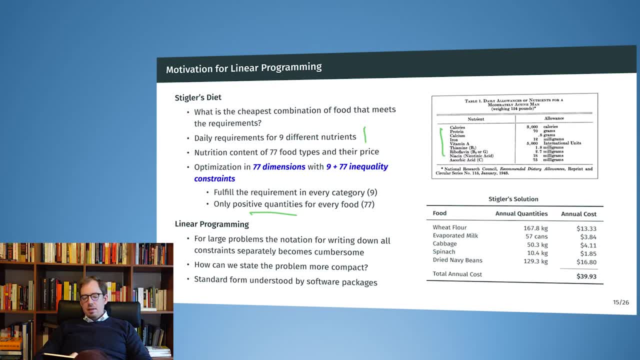 so for large optimization problems- and now we are still- this is still tiny. so now we are 80 dimensions, 80 something dimensions. this is still a very small problem, but it becomes problematic to write it down by hand and we don't want to spend weeks and weeks doing the calculations by. 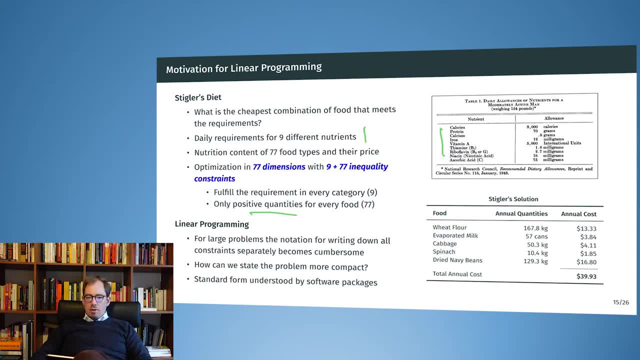 hand. we want to solve this by the computer, but even when we think about the problem on paper, we'd like to have a shorted, shorthand notation that states the problem a bit more compact and where we still have a good way to think about and reason and talk about the problem. 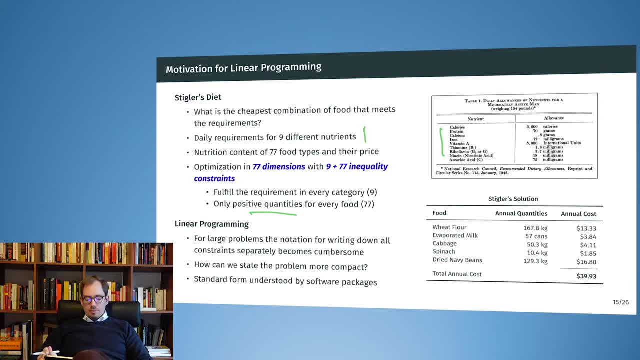 with a with a compact notation, and also linear programming is not only a shorthand notation, it is also a standard form understood by many software packages. so it's a standard way to express a certain type of optimization problem, and then i can choose between different algorithms that all understand the type of of problem definition. 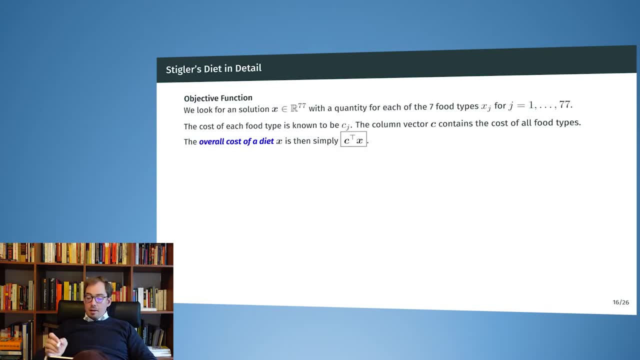 okay, so stickless died in detail. for the objective function, we are looking to minimize the cost of the overall diet. so let's assume we know the cost of every food type and the food type is here indicated by, by j as an index. so j is between 1 and 77 and we know the cost of every food type. 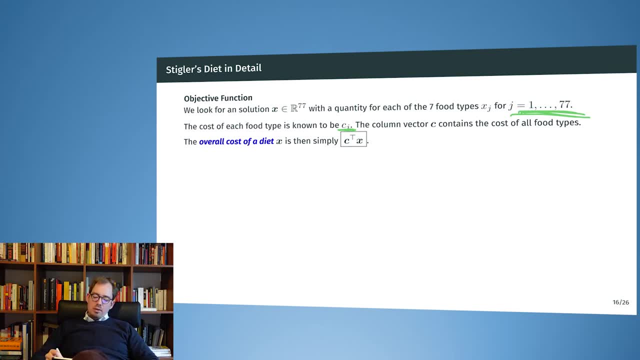 and we put the, the c, j together to a vector. so we have c1, c2, c3 and so on in a column vector that contains all the, the cost for the different types of food. meaning, when we then have decided on an overall diet, x that contains the number of food for every category. so here x would then also be a. 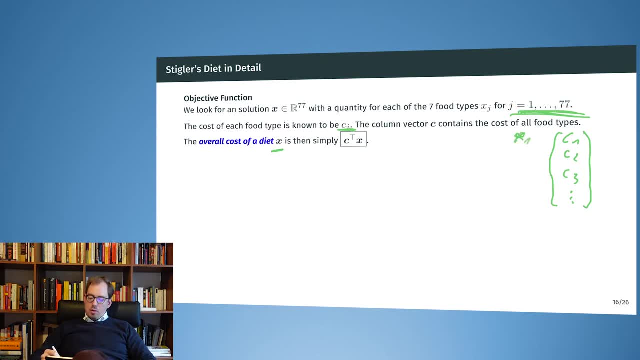 column vector where all the entries correspond to the different food types, then the overall cost of this diet would be just c transpose x, so we transform c into a row vector. multiply that with x and this little expression here. this is the objective function that we are minimizing and this is actually a what is called a linear. 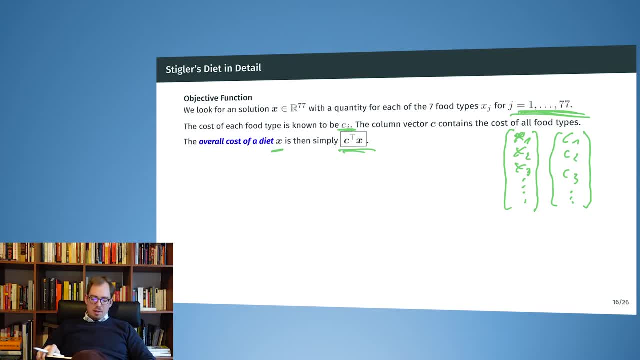 objective function. so one of the simplest types that we can have. okay, now, in addition, we have the constraints for the nutrient requirements. so for all the nutrients, we know how much. we know how much food they they contain, how much. for every food, you know how much nutrient it contains. so for every type of nutrient, 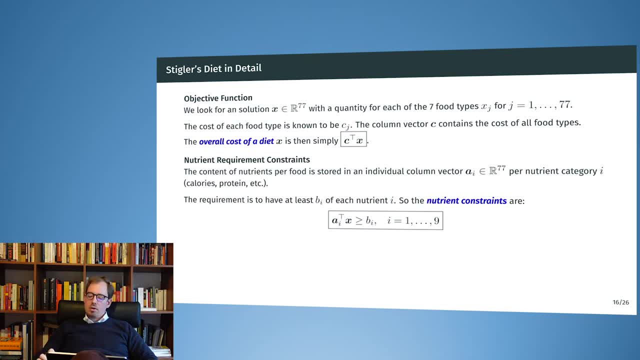 so we have different nutrient categories and the nutrient categories are called I here. for every category we have again a column vector that contains the number of nutrients for the different foods. so up before we had a column vector that was also for the cost, that had 77 entries, so with one cost for every type. 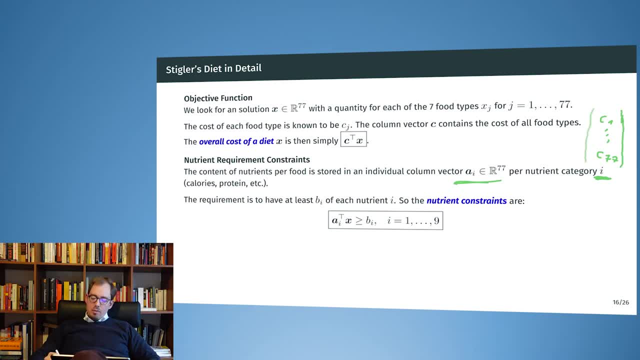 of food, it now for the nutrient contents. we would then also have a 77 entry or 77 dimensional the vector, but then we have have a different vector for the calories. so we have one here for the calories and then maybe another for the protein, and for each of the types of food we have a. 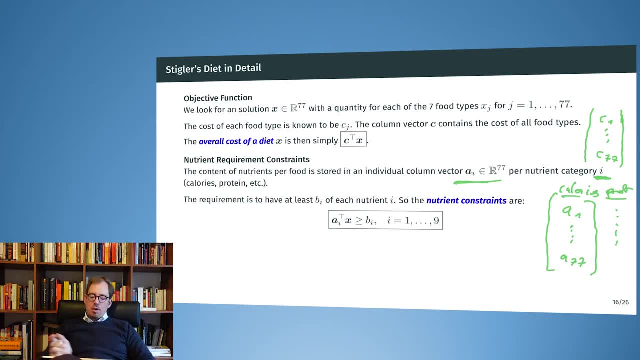 different column vector that describes the nutrient per food type. okay, and now we can formulate the constraint. so now we say AI transpose X has to be larger than bi and the bi is the minimum requirement for the nutrient type I. okay, now moving on positivity constraints. these are rather straightforward, so I 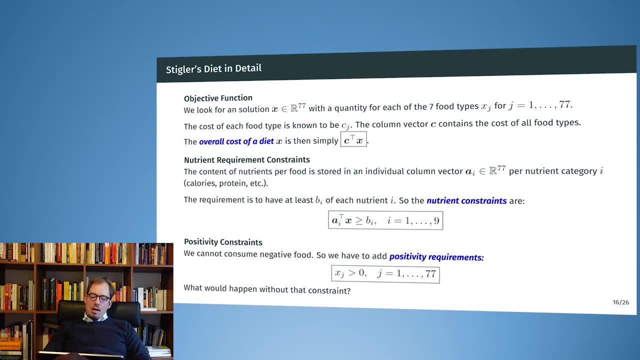 have 77 food types and I just add the constraint X, J, larger than 0, and so overall I have a linear optimization target function. I have 9 inequality constraints for the nutrient content and I have 77 again inequality constraints for the positivity and this makes up the optimization problem of Stigler's diet. 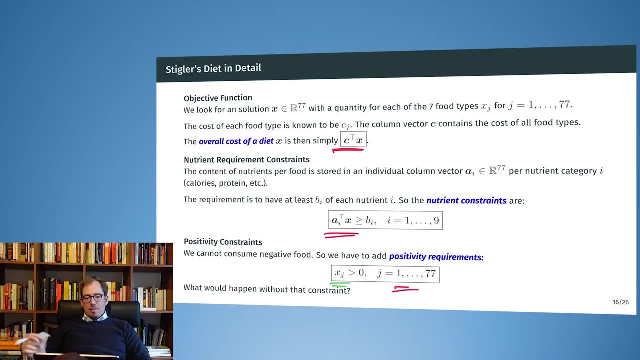 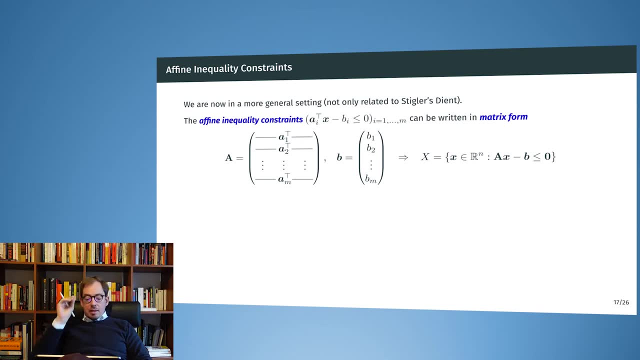 and now we compress this even more and right bring it into standard form. so now we rewrite this by taking all the inequality constraints and and putting them into a matrix form. so we have just seen the constraints for the different types of food and when we rewrite this constraint. so here we. 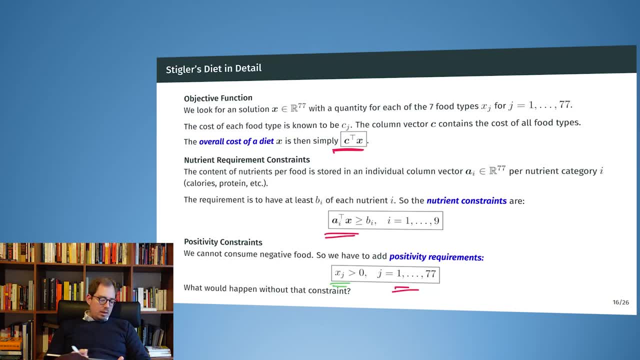 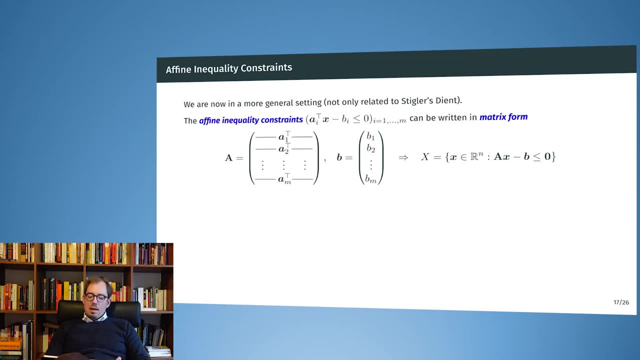 are looking at this, this constraint here, and when we rewrite this, we can write it down as AI transpose times X minus bi has to be smaller, equal than zero. so again here we are, in standard form, smaller, equal than zero. and if we, If we then take the AI and transpose them, then we can stack them on top of each other. 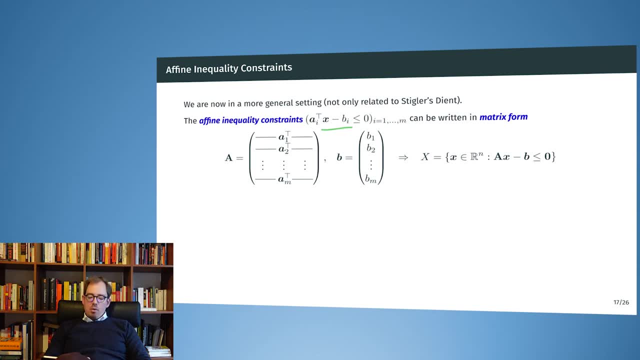 to form a big matrix A, And every row of this matrix A then contains one inequality constraint, And then prior we had to consider all of the inequality constraints individually, but by putting them into this standard matrix form we can just write down our solution, set as: 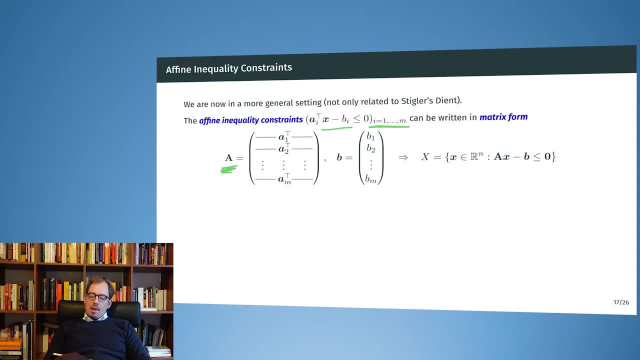 all the solutions X, where A, X minus B is smaller than zero. And now big A is a matrix and X and B are vectors, And obviously I'm modifying my X here and I'm looking for all X where this equation holds for a known matrix A and a known vector B. 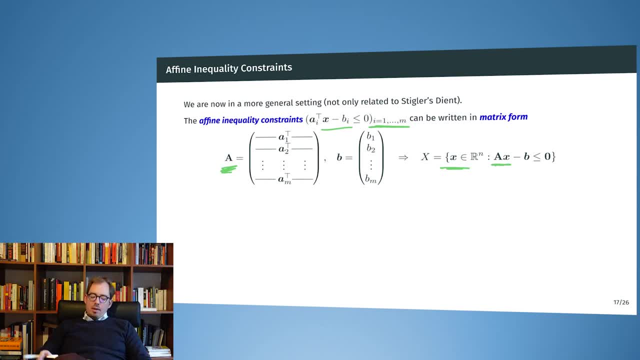 Okay, And for the Stigler's diet we had all the AI. So the AI were from the notation. we reused the A notation here Previously. these were just the nutrient constraints, but also the positivity constraint for every food type can be expressed in a similar way. 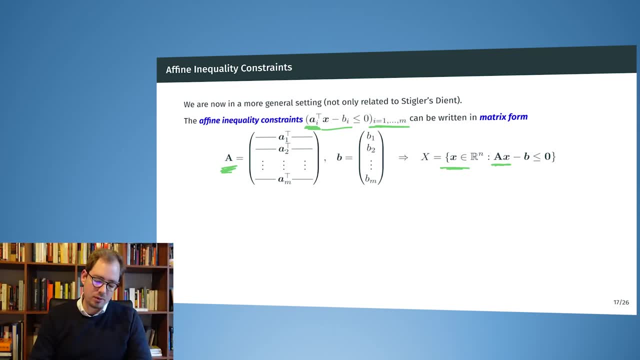 So I could. for the A I could just have a matrix, For example, where I put only one entry here, So one one, and otherwise I only have zeros, And in that case if I say A X minus B is smaller than zero, and that would mean X one minus B. 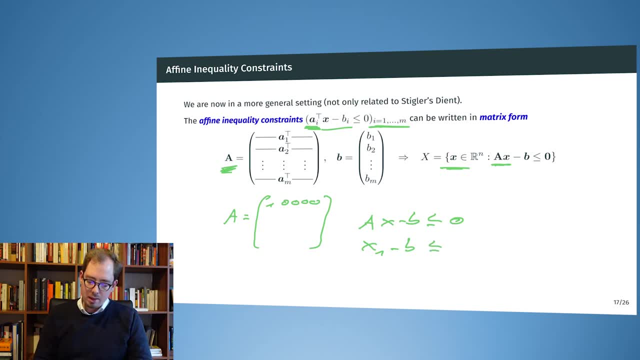 smaller than zero for for the first row, So B one, of course, the first element of B. So now, looking only at the first row of this guy, it would then be equivalent to the constraint X I smaller than B I, And that way I can just express the positivity constraints of the Stigler diet. 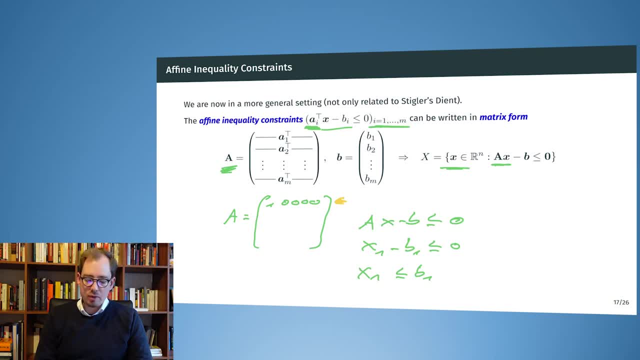 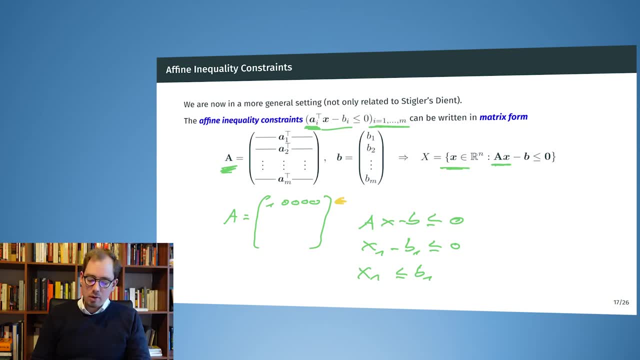 into into one simple expression, Because now, overall, um, my optimization problem it looks like this: Um, I minimize F of X subject to A, X minus B smaller than zero, And this is the compact form for for linear programming. 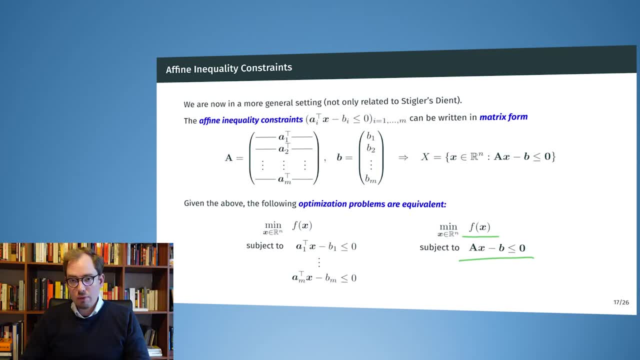 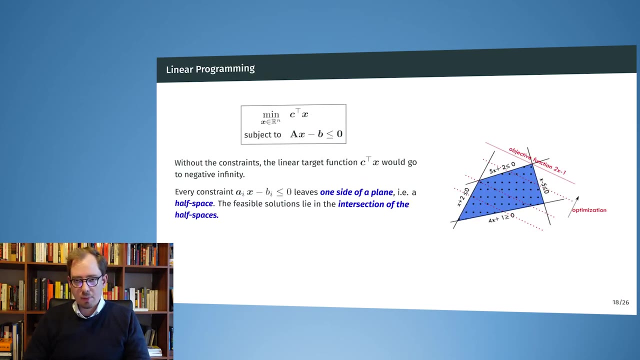 Okay, This was quite a bit Uh. you will also solve Stigler's diet, or a variation of Stigler's diet, for yourself. So this will be a problem for the for the exercises, Um. but now let's um look at a little more at what uh linear programming uh does and how. 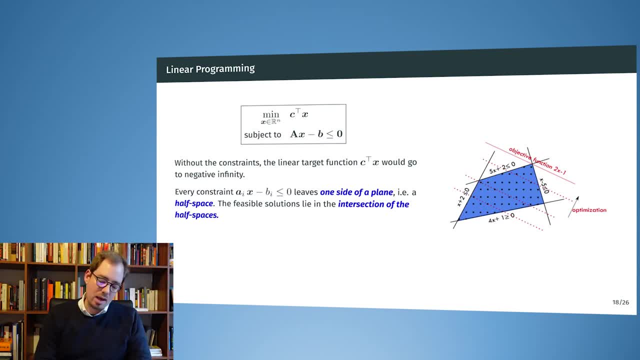 we can visually think about linear programming. Uh, we have, uh, our linear problem, C transposed X that we want to minimize, and we have our constraints. and every row of my matrix and every entry of the vector B now defines a, a, a, a a. 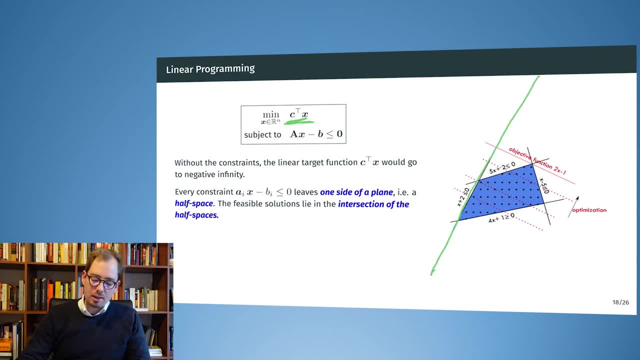 plane in The solution space and it is excluding a half space. So all the blue points here are all the shaded area here would be excluded. And again I do that many times, um and uh. take the intersection of the remaining set. 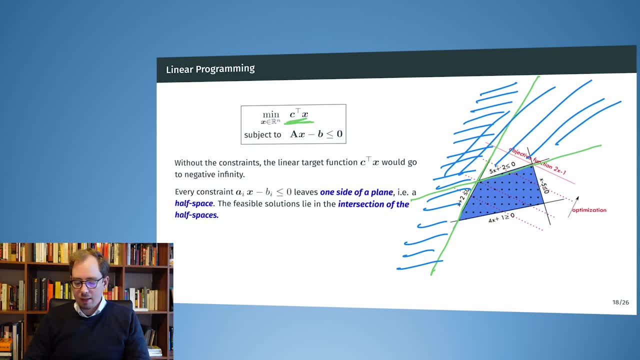 And uh, then I get like a polytope and all my uh results have to lie in that polytope. Uh, in this case, here the The solution set is closed on on every side. Uh, but I can also imagine an example where I have- um, let's draw this differently- where I have uh, 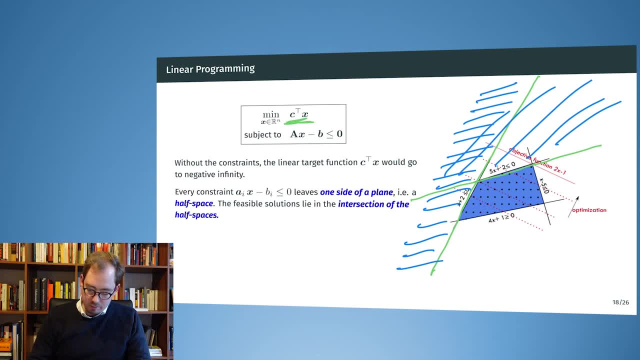 Okay, Where here I have uh X1 and X2, and my constraints are, for example, that: Uh X1.. Uh X2.. Uh X3.. Uh X4.. Uh X5.. Uh X6.. 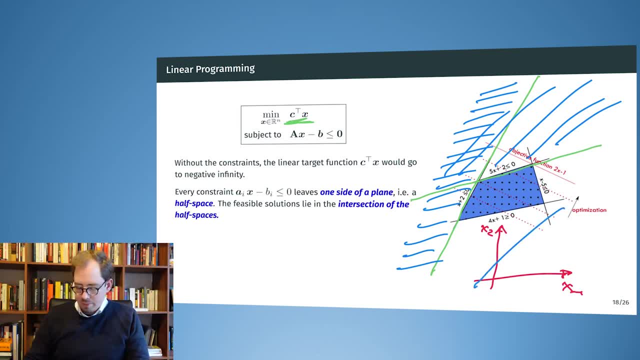 Uh, X7. Uh, my solution, uh, has to be outside of the shaded area, And then my solution set would be open. So then on, on this end, here, my solution set would be unconstrained, And I could walk out to infinity over there. 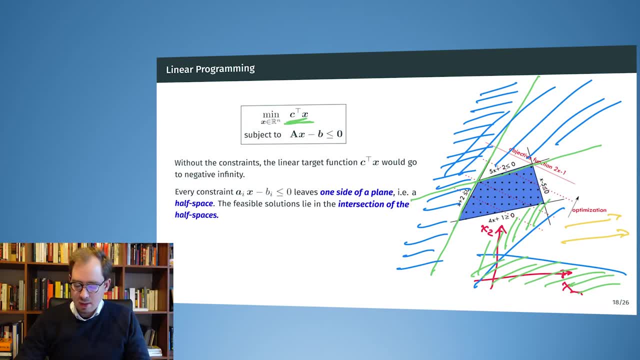 Uh, but I, I won't have a problem in that case If my, If my optimization problem forces me inside the barrier. So for the, for the linear programming, um, if, if, I can, I would walk infinitely, uh, far along in the direction where my solutions are getting better. 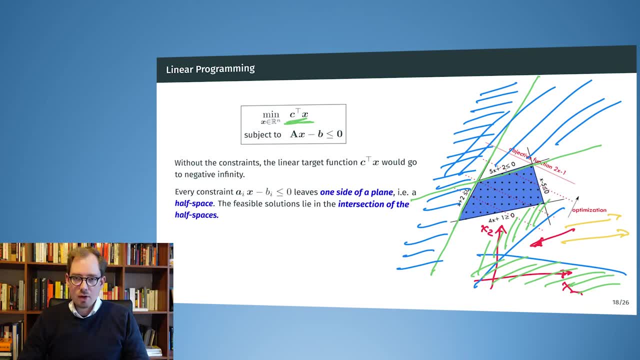 Uh, so for for linear programming, I actually do need the constraints. Otherwise, if this was unconstrained, if I only had C transposed, X as the optimization, with no constraints, then I would walk straight out into infinity If I'm not on a, on a, on a exactly flat line. 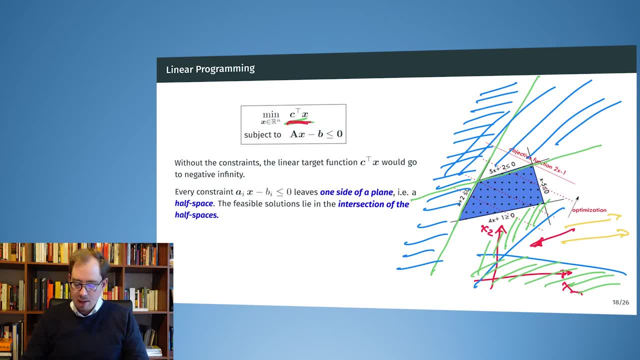 And uh. therefore, I need the constraints to have a well-defined solution And I also need the optimization problem to walk in into the constraints. And uh but uh. this is often designed into the optimization problem. So when we state the optimization problem, we already have. have that in mind. 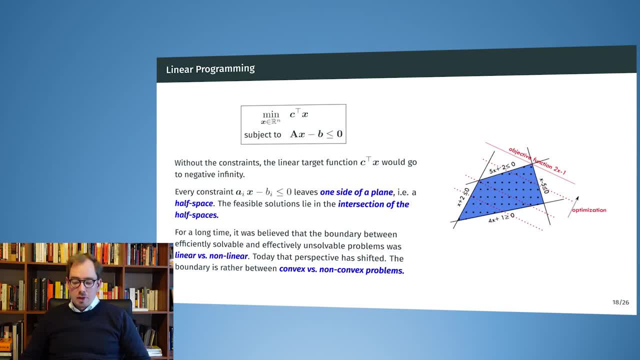 Okay. So for a long time it was believed that the boundary between efficiently solvable problems and, uh, very complicated heart problems, uh, was the difference between linear and non-linear. Today, we rather believe that the boundary is between convex versus non-convex problems. 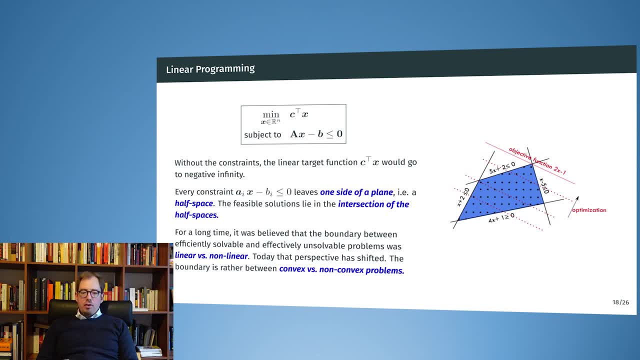 So today we say that the convex problems are efficiently solvable and the non-convex problems are not efficiently solvable. but for many years, until, let's say, The the late 80s, even in many circles it was believed that the linear problems, only the linear problems. 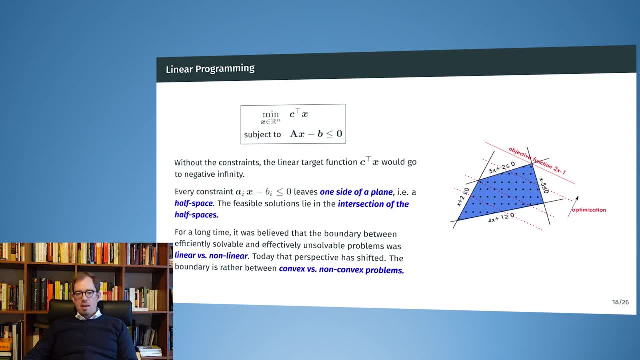 were efficiently solvable. today we are a bit further than that. today also, many convex problems that are non-linear can be solved efficiently. but from a historical perspective the linear problems are very important. many practical applications can make use of that. they don't require non-linear optimization, but also the the solution methods for linear problems have. 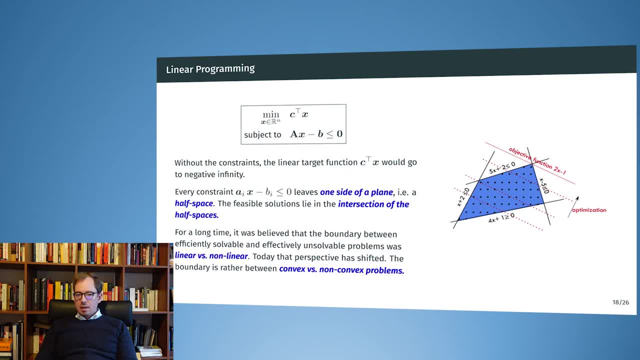 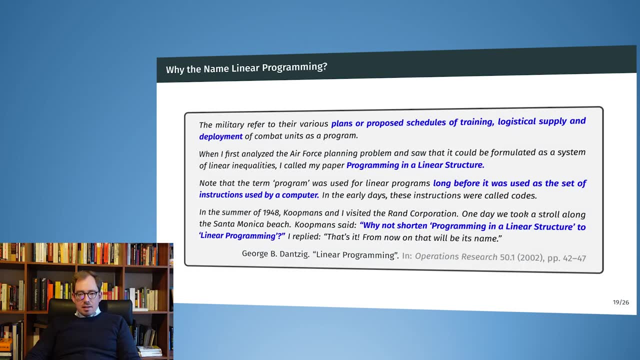 were the first to reach a level of maturity where, on an industrial scale, the the methods could be used. okay, where does the name linear programming come from? so if you are students of computer science, so most of you you will understand programming to be the development of computer code, of program code. but linear programming is obviously something very 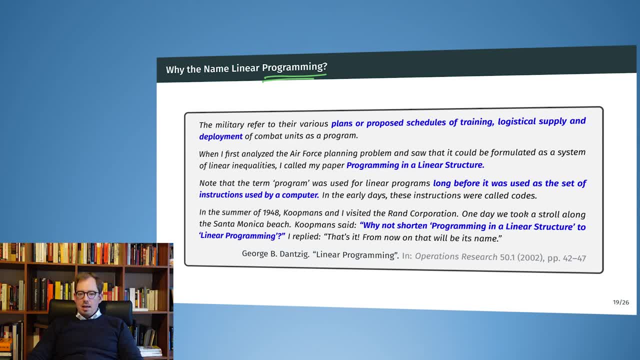 different. but why this overlap in naming or this name confusion? well, actually the programming term for linear programming is much older than the programming term for computer programming. so originally the military referred to plans or two schedules for training, learning, logistics, deployment of troops and so on as a program and the this optimization of the programs. 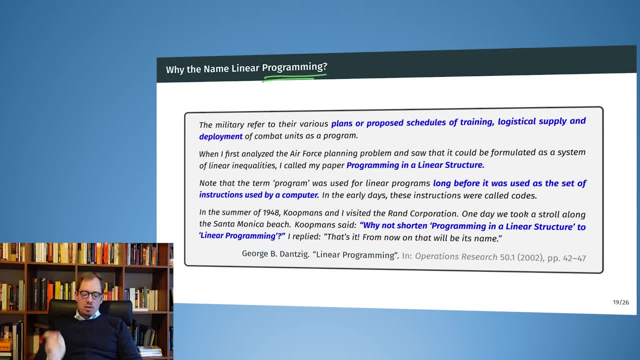 of the military, was one of the very first applications for the, the tools that we are today called linear programming, and for the type of problem that we today call linear programming and judge dancing, which is one of the grandfathers of optimization. he he first called this approach programming in a linear structure and later on, a colleague of him, 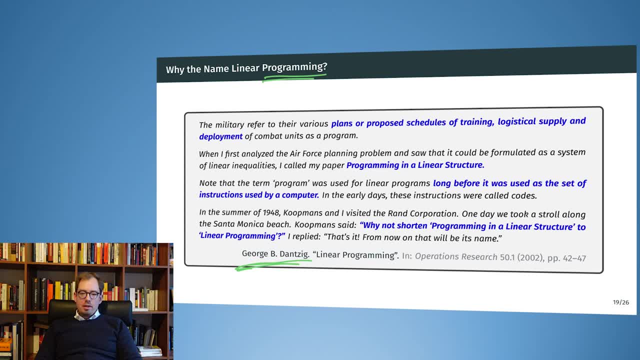 cook months. he proposed to shorten the name to linear programming, something more catchy in science sometimes. sometimes you want, you need your science to have a sexy name to to catch on, and in that case linear programming did take on and today it is the term used to use the term linear programming. 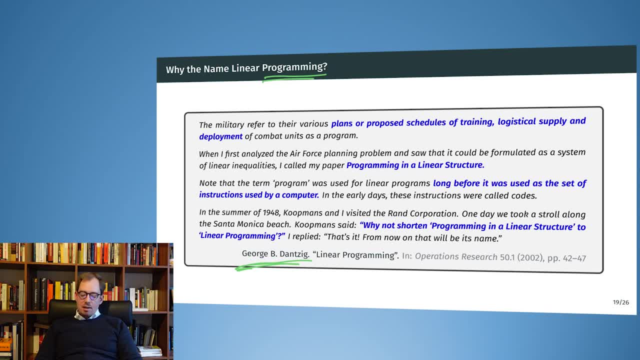 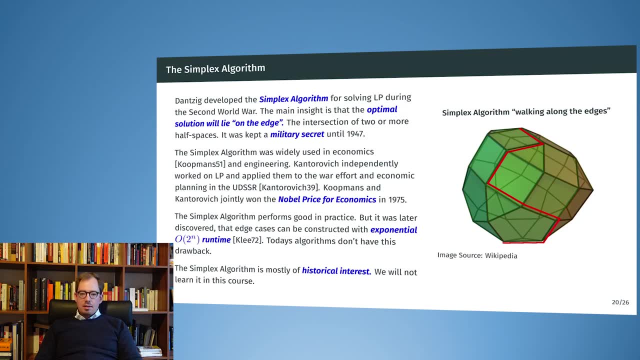 for the type of problem that George dancing has been solving. at the time, well, judge dancing was also the inventor of the simplex algorithm and he developed that during World War two, and actually the military kept the algorithm secret until 1947 and it was then published in in the 50s. 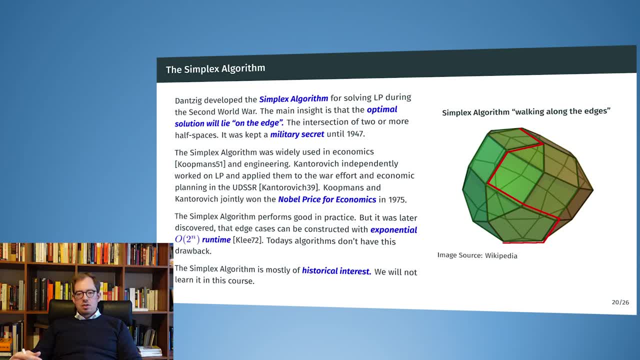 because it was such important, of importance to the war effort, and they wouldn't want to leave this algorithm to optimize the military programs to the enemy. Okay, so what does this simplex algorithm do? How does it work? The inner workings of the simplex algorithm are much more tuned to linear programming, So the 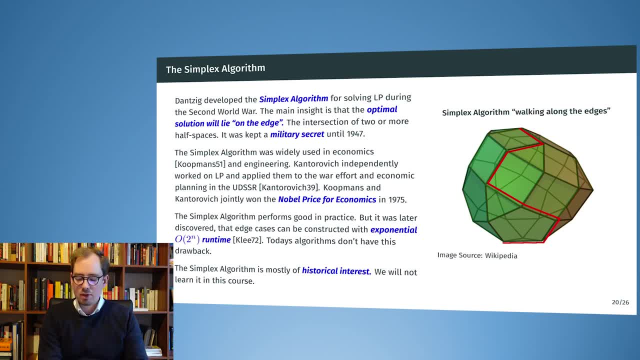 barrier method that we saw earlier, the interior point method that we saw earlier. it can be applied to a wide variety of different problems. So the resource allocation problem that we solved early on in the lecture, this was already a nonlinear optimization problem, but the simplex algorithm only works for the linear optimization problems and 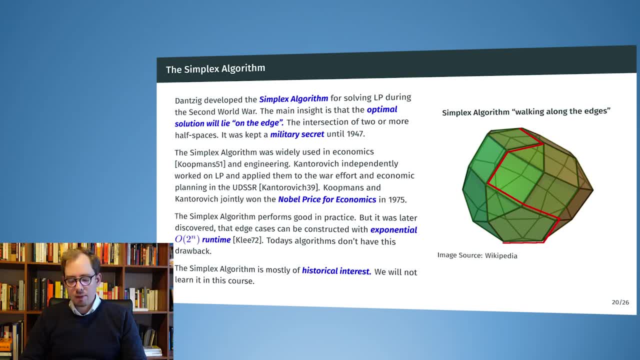 it exploits the, the approaches to the Darumer создAS cooling method And this can really help that. the insight that the solutions will always lie at the intersection of several constraints. Well, I have to explain that a little bit. If I have a constraint that is exactly orthogonal. 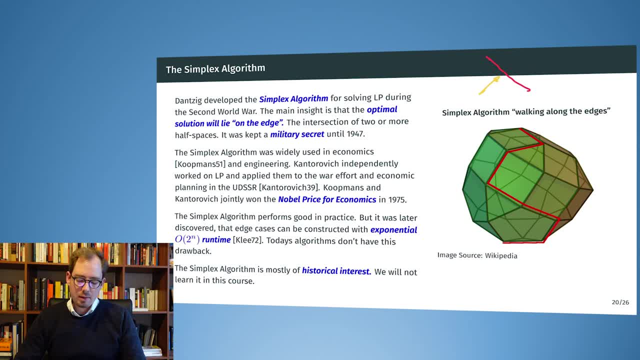 to the direction into which the optimization objective function is forcing me, then the actual solution can lie on all the points here, on this line or on this plane in a higher dimension. But if I have a search direction that is not entirely orthogonal to the constraint, 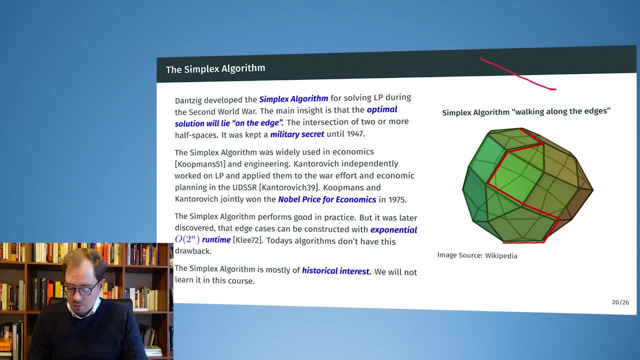 then. so this again is the constraint, and this would be my search direction. then I would move over here and here and here and get better and better and better until I walk into another constraint. So I am now excluding all the solutions outside here and the optimum you can imagine. 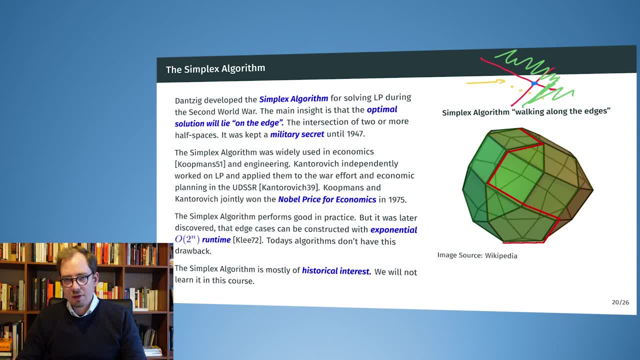 the optimum has to lie, then, exactly here at the intersection of these two constraints, And the idea of the simplex algorithm is to walk along the edges and to take a direction or to select the next edge in a way that I'm always improving on the solution. So here we. 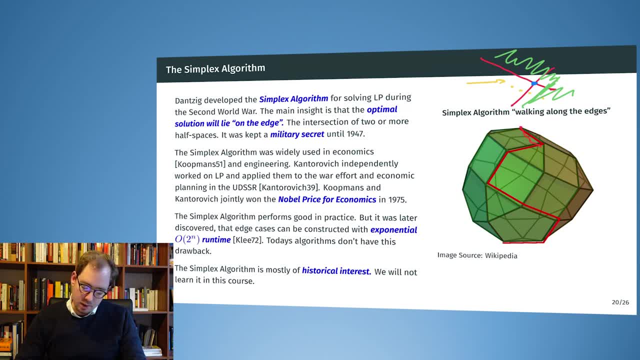 are starting starting at some point: walking over to the next vertex along the edge, walking over, walking over, walking over and the simplex algorithm. it defines a way to select the next edge and there are. you can even do that on paper for smaller problems and this has a big impact and for for a big part of the 20th. 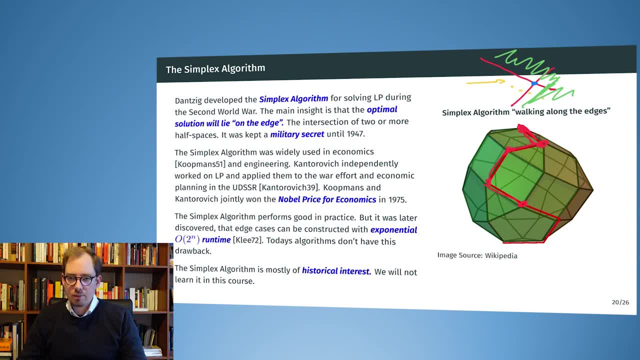 century. this was heavily used in industry and military context and so on. People won Nobel awards for that. So for example, Kopman's, which was mentioned on the previous slide, and also Kantorovich- they defined important optimization problems in economy and jointly won the Nobel. 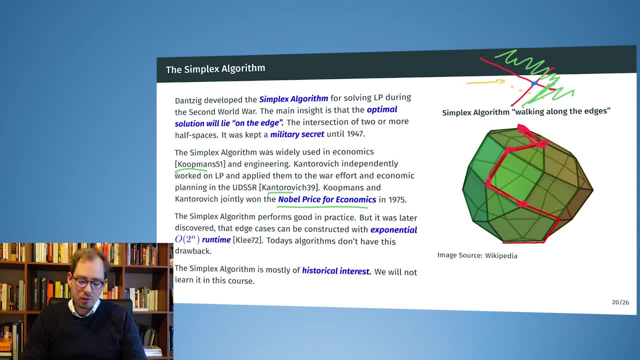 prize for economics in 1975.. And Kantorovich, for example. he was famous for employing the optimization methods in in Russia, in the UDSSR, to optimize the economy on a state level. used for for economic planning. Okay, the simplex algorithm. why are we not learning about that here? 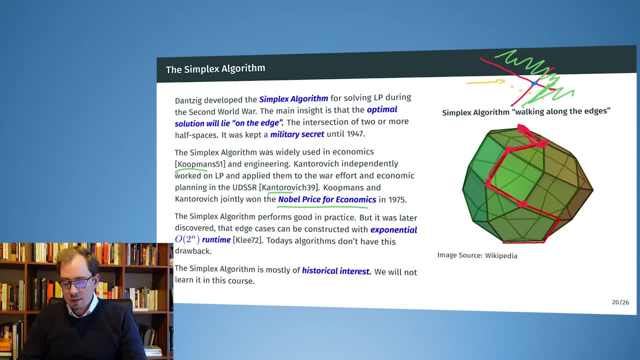 in this lecture. First of all, it is constrained to the linear programming case and we are looking at a much wider class of optimization problems here. and also, it was found out in the 70s. so Klee is the author here. it was. it was found out in the 70s. 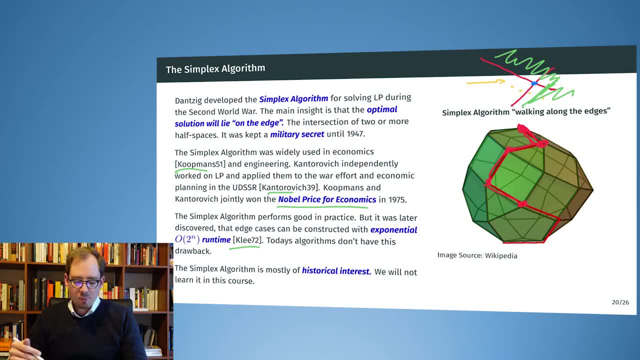 that we can construct synthetic problems where the simplex algorithm has an exponential runtime. So this rarely occurs. this rarely occurs in in practical problems. but by carefully constructing the problem we can. we can have exponential runtime and this is a drawback because we don't have any guarantees. So sometimes your algorithm 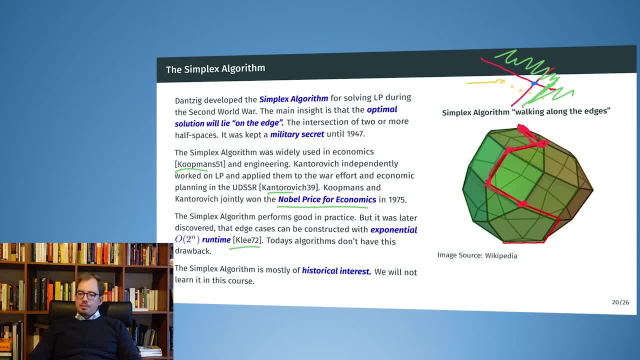 it needs a guarantee to converge within a certain time or to get to get to a good enough solution in a certain time. so, for example, in a safety critical context or in an automatic, automatic control problem, you want to be able to, to, to guarantee that within I don't know a tenth of a. 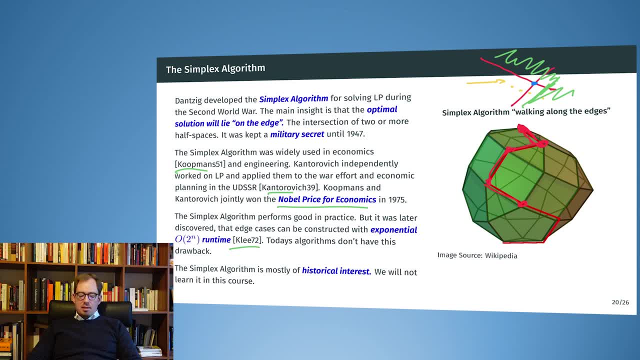 second, you have a good solution and with the simplex algorithm you cannot the the bounds you get from the run time are pretty bad, because it could always be that you run into a case where the runtime is exponential in the number of the constraints and the variables, and today's algorithms don't have this drawback. 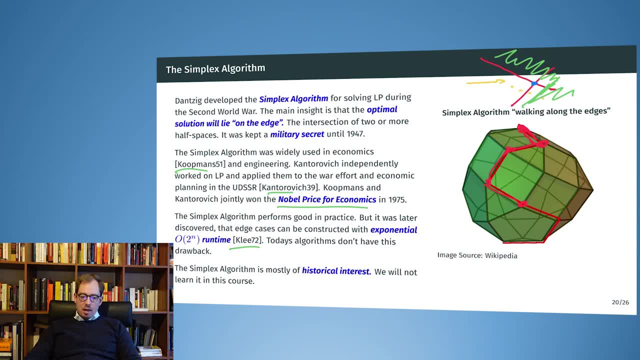 and today's algorithms have reached or even surpassed the average runtime of the simplex algorithm and they generalize to also to the non-linear problems and they don't have the drawback of the exponential runtime. so it was in the in 1988 some some researcher at IBM. 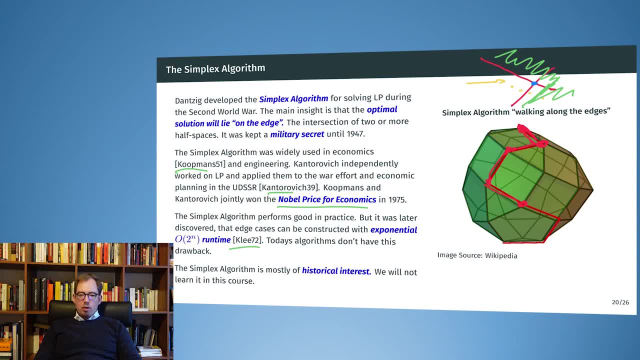 published the first algorithm that showed polynomial runtime for the, for the linear programming problem, or the first polynomial runtime that was acceptable, and this triggered a big again a big revolution in the optimization field. The problem then was Karmaka was the name of the researcher He patented. 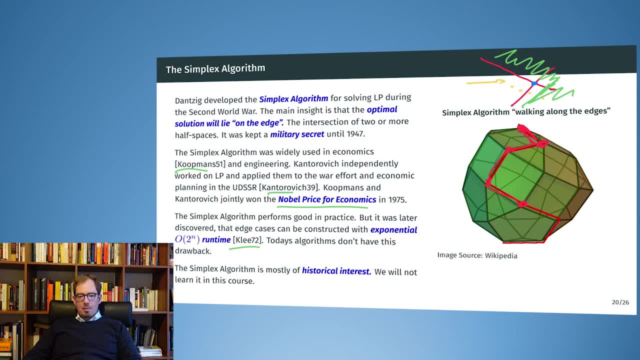 his algorithm and uh, so IBM and Karmaka patented the, the approach, and uh, but within within month and the first year, people found improvements that were no longer covered under the patent, and today patenting is is no longer a problem. in the field of optimization, Okay, but the, the simplex algorithm, that that